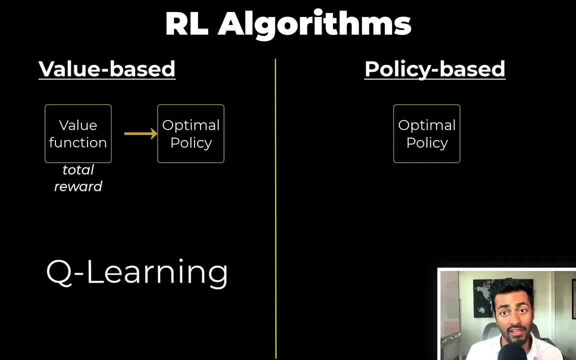 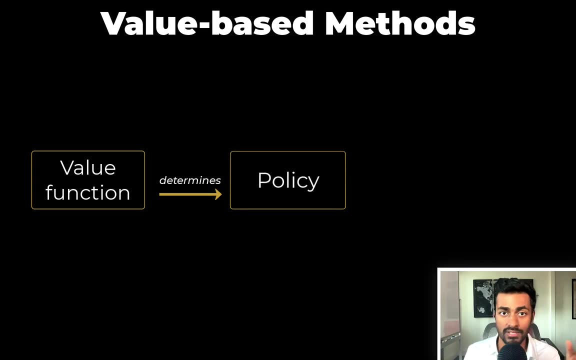 or state Now: Q-learning is a value-based reinforcement learning method to solve problems, And so we can dive a little bit more into these value-based methods. So value-based methods determine a value function that in turn determines a policy that's going to maximize total rewards. A value function is a function, So it has some. 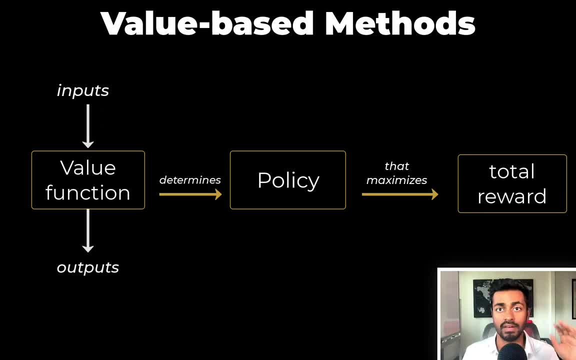 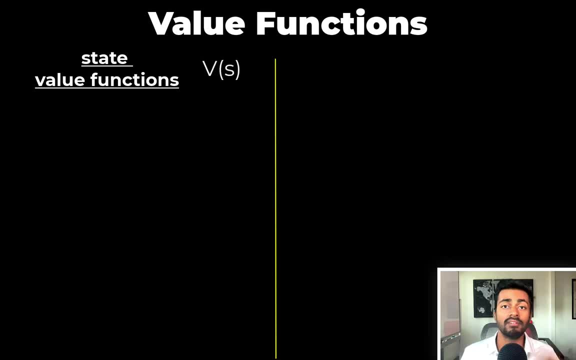 inputs and it generates an output. And depending on the inputs, there are two types of value functions. We have state value functions, represented by V, And then we have state action functions, represented by Q. But now states actions, what are those? A state is a snapshot. 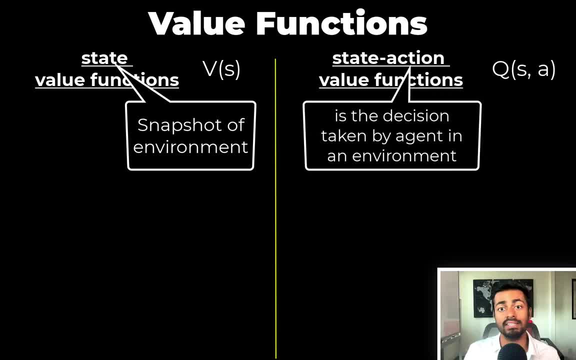 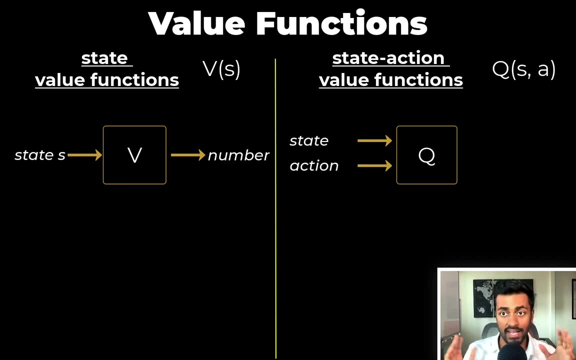 of the environment And an action is the decision taken by an agent in an environment. So the state value function will take a state as input and output a real number, Whereas the state action value function will take the state and action as input and it'll output. 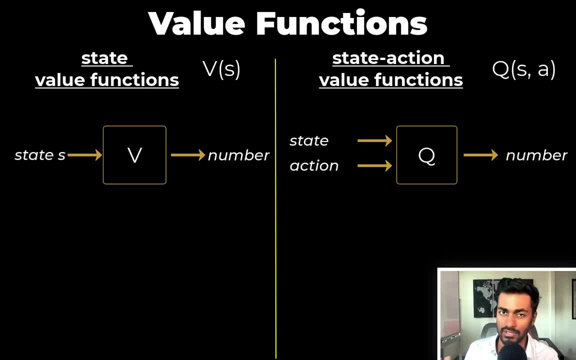 a real number. So this real number is also known as a Q value. Ooh, Q. So we're getting close to Q-learning here. Now the state value, that is VFS, will quantify how good is it to be in a given state S, Whereas 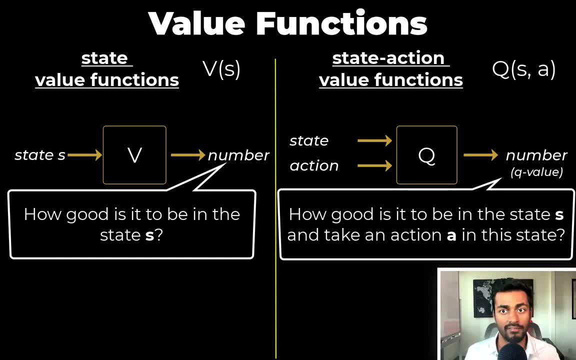 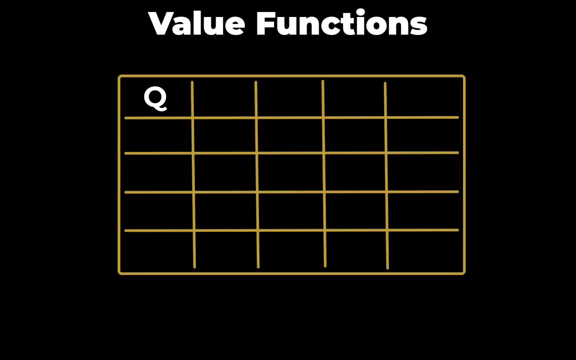 the state action value, or Q value, will quantify how good is it to be in a state S and then take an action A in this state. For Q-learning, we are interested in learning the state action value function Because it's a function. you can think of it more easily as a table of rows being states and columns. 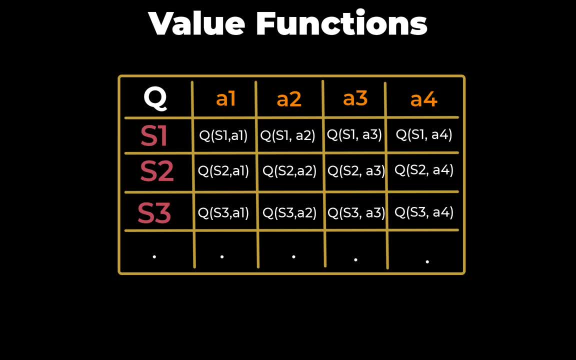 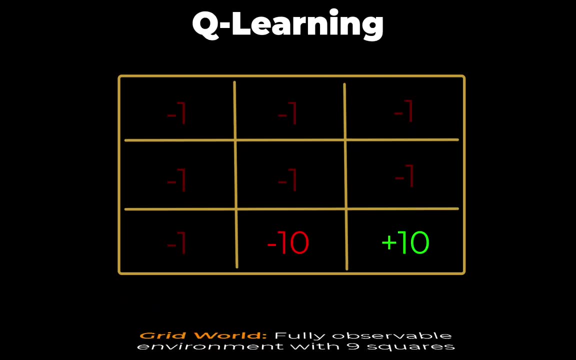 being possible. actions And each cell value will actually be the Q value for that given state and action, And the goal of Q-learning is to effectively learn these Q values such that the total reward is maximized. So let's see how it works with this grid world. So this here is a fully observable environment. 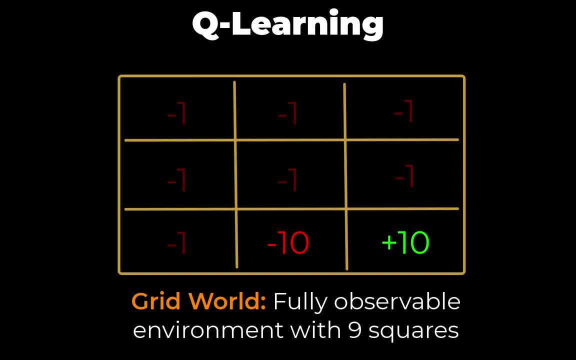 with nine squares And there's a plus 10 reward square, a minus 10 poison square and other rewards is negative 1 for any other square. Now the goal of our agent is to get to this plus 10 reward spot in the best. 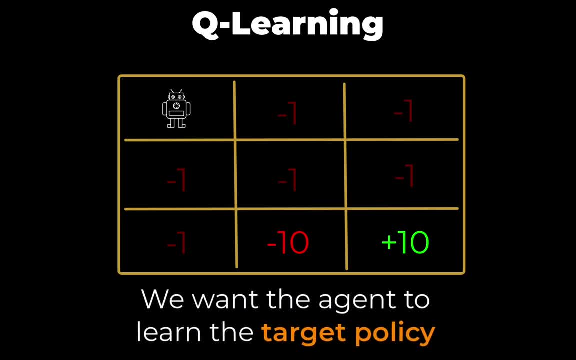 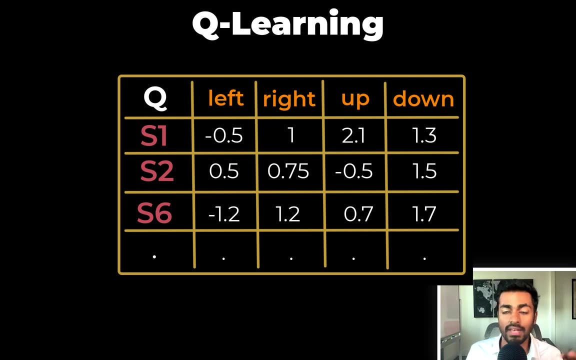 possible way, And, more technically, we want the agent to learn an optimal policy. This is known as the target policy, And let's say that, in order to learn this optimal policy, we want to use Q learning to do this, And so we need to make use of this Q table. Let's initialize these values to: 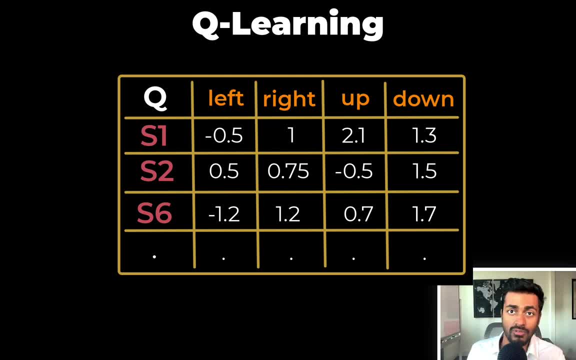 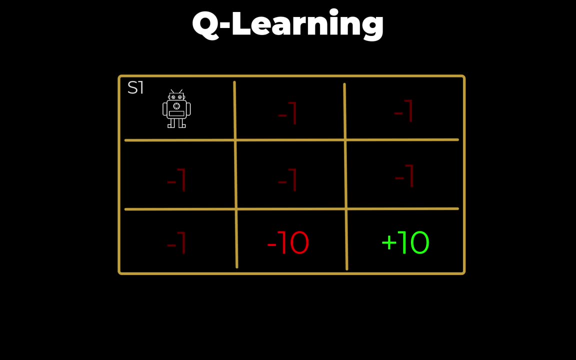 arbitrary values. Now note that these values could also be loaded by some other agent that explored the environment previously, But for now let's just keep them arbitrary. Now let's say that the agent starts in the first cell at state S1, and it takes an action based on exploration policy. 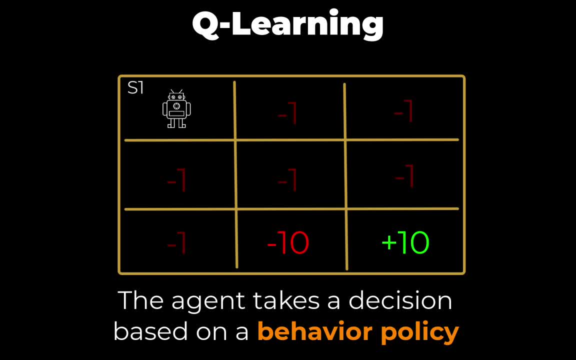 This means that the actions that an agent takes is simply based on random chance and the agent won't just choose a state because it has a high Q value, for example. And this policy is known as the behavior policy, And it can be just about anything If the agent is in a state S1,. 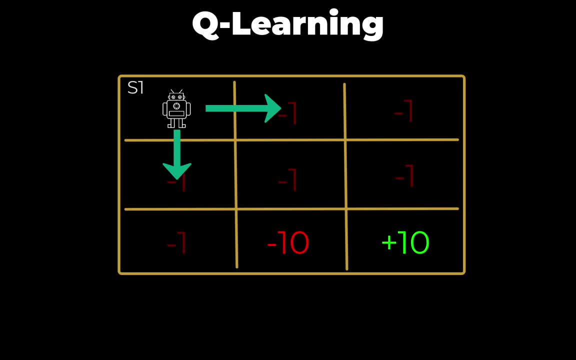 it can take an action of either going right or going down. And because the policy is random, let's say that the agent made the decision to go right, So the action is taken, And then, when taking the action, the agent transitions into another state, And let's say that this another 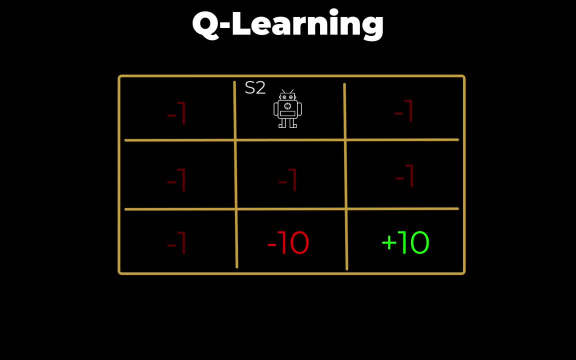 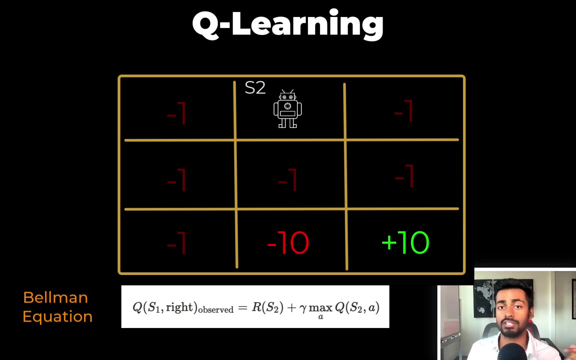 state is S2.. And on doing so, it also receives a Q value, And then, when taking the action, it also receives a reward of negative one. Now let's calculate the observed Q value. So this is given by the Bellman equation. Now, the Bellman equation defines a recursive relationship between: 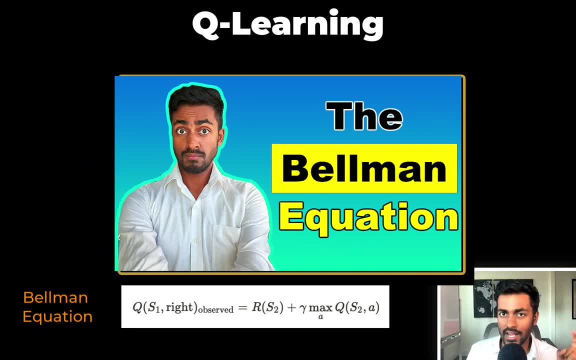 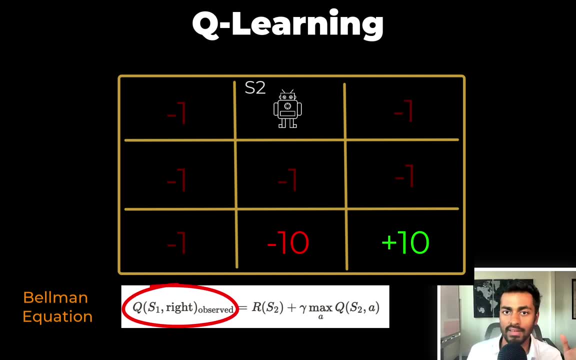 Q values And for more information you can check out my video on the topic. But for now the Q value for the state S1 and right is given by the sum of the reward of state S2. Plus the maximum future Q value for that state S2 that we can get, And gamma here is a discount. 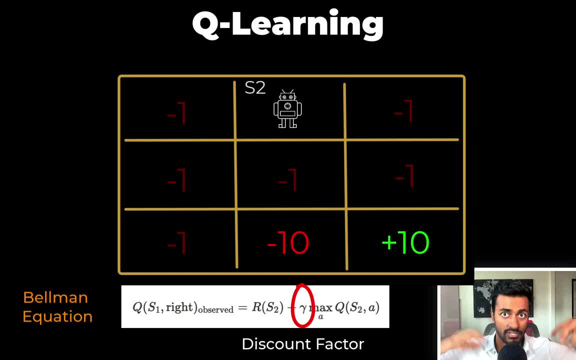 factor just to show how much we want to value the current reward over future rewards. And so if we just plug in some values, so the reward from S2 is negative one, let's say that gamma, that discount factor, is 0.1. And then we multiply that by the maximum possible Q value that we can. 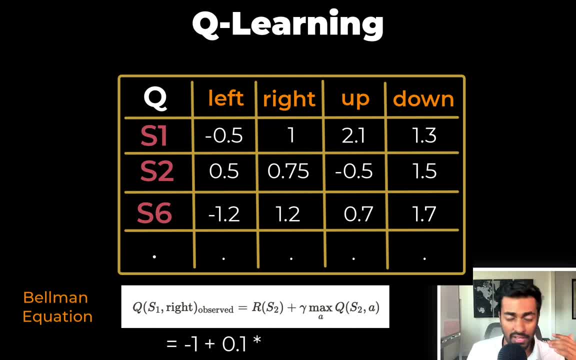 get from state S2.. Now, looking at our Q table, we can see that we get the maximum Q value by going down from the state S2, which is 1.5.. So substituting 1.5 in our equation, we'll get the. 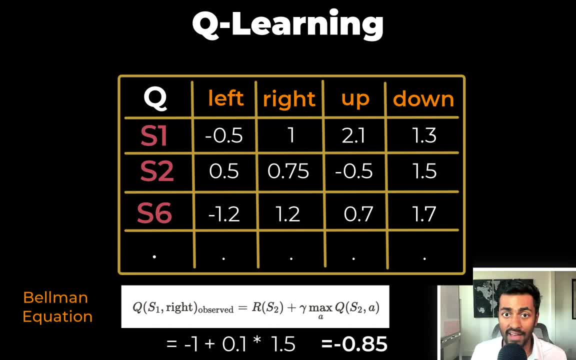 overall Q value as negative: 0.85.. This is the observed value for Q1, state S1 and going right, But the value at the table for this specific Q value is one, But it's clearly a difference and this difference is an error. that is known as a temporal difference. 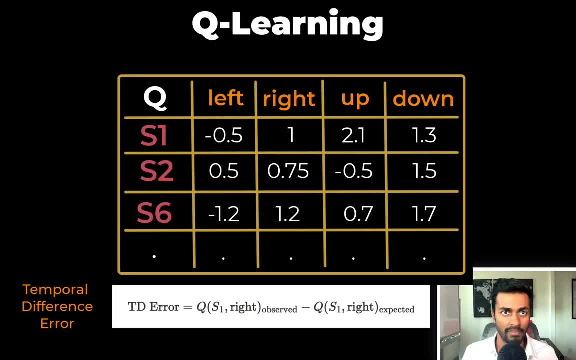 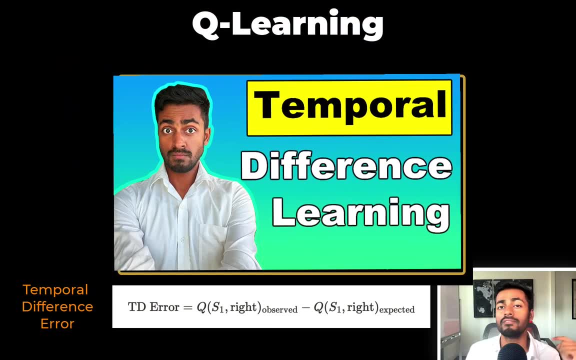 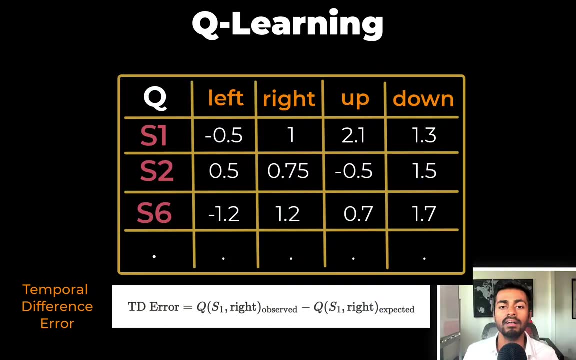 error. It's called the temporal difference error because we are comparing Q values of two different time steps and their difference is the error. hence the name. For more information on this topic, I created another video right here, But for now, temporal difference error is now going to be the observed value minus the expected. 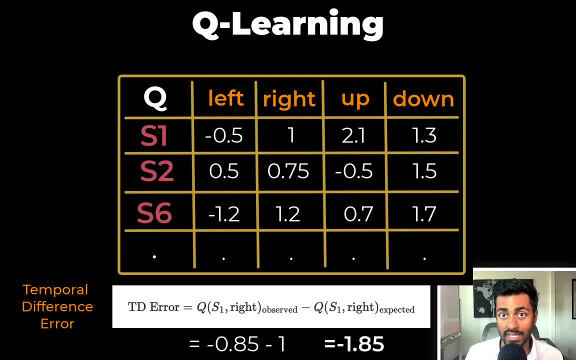 value, which will turn out to be negative 1.5.. So we're going to go ahead and do that. So let's give 1.85.. We now update the Q value in the table based on the formula that looks like a gradient: update rule. 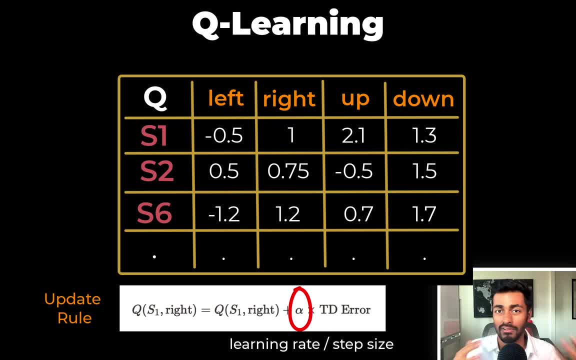 And here alpha is going to be the step size, or the learning rate, so to speak, and it defines how much in every time step are we willing to change these Q values. Higher the value, faster learning, because bigger the updates. So in this case let's also just take it to be some 0.1. And plugging in 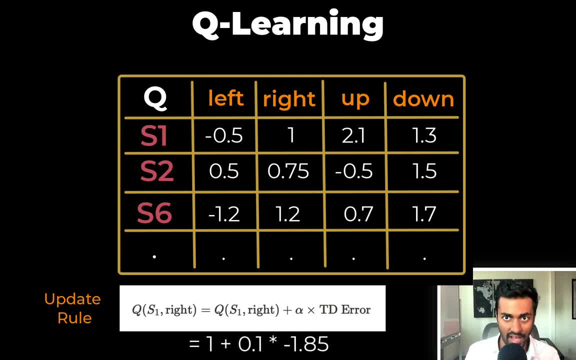 the values, we get one, which is the expected value, plus 0.1 times the error, which is negative 1.85.. And then, doing the math, you will get 0.815 as the final result, And so we update this single. 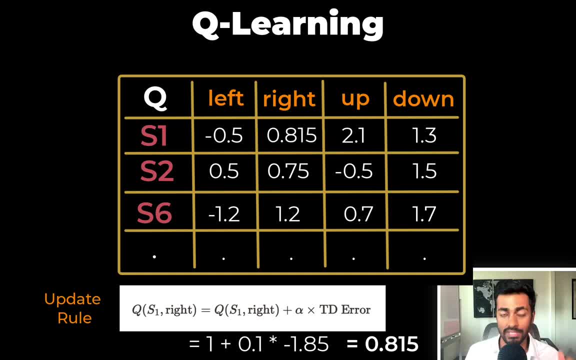 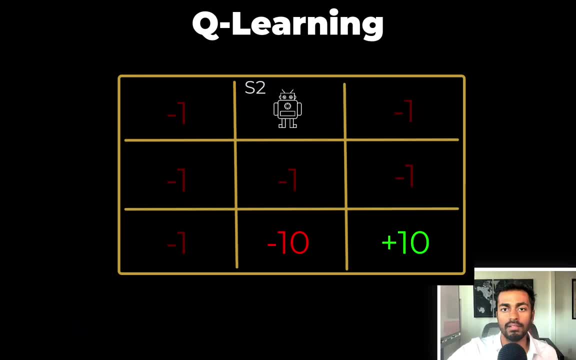 Q value in the table from one to 0.85.. And this is the end of our first time step. Let's now walk through another time step, just to make sure that we understand what's going on. So let's say that now we're in a state S2 in time step 2, and we can take the action of either going. 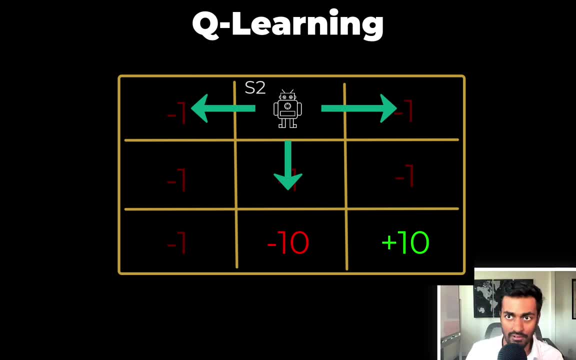 right, left or down, And the policy we are following is now random. So let's say that we choose to go down, We take the action and then, on taking the action, the agent will transition into another state- Let's say it's S6, and it receives a reward of negative 1.. Now let's calculate. 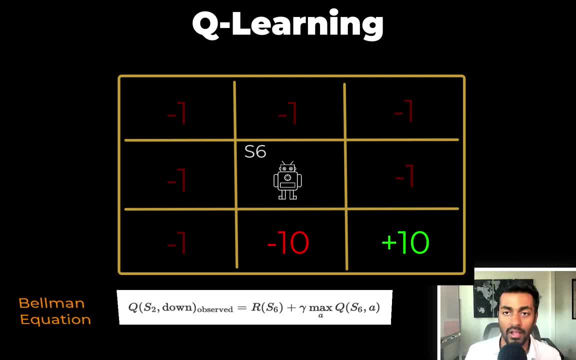 the observed Q value that is given by the Bellman equation. So the Q value observed is going to be the reward in transitioning into state S6, plus the discounted maximum value that we can obtain for state X6. And so we know that the reward for state S6 is negative one, And from our table 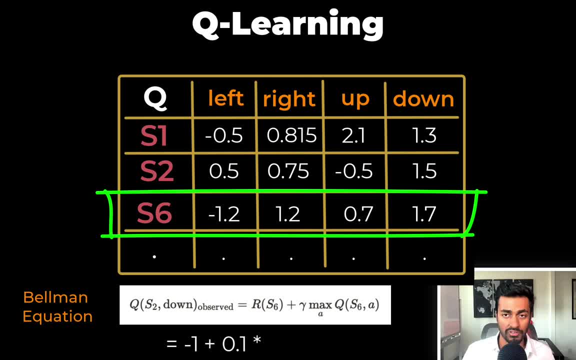 when we are in state S6, the maximum possible Q value is going to be 1.7. And this is the value where we're going to take that constant value from G and do that via Q announcement from inside S6. So we're going to take that constant value from G and we're going to take that constant. 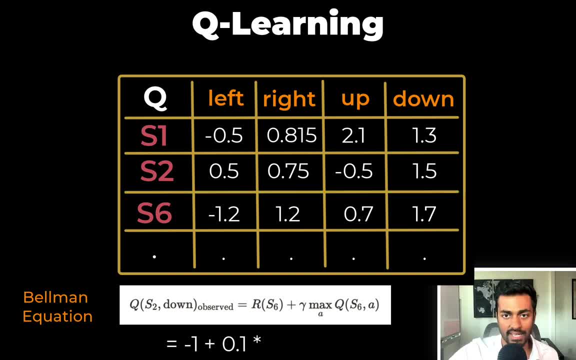 value if we choose to go in the downward direction from S6.. So we substitute that in the equation and we get negative 0.83.. Now this is the observed value, but the expected value that is stored in the table for this cell is 1.5.. And so the temporal difference there is going to be the difference of. 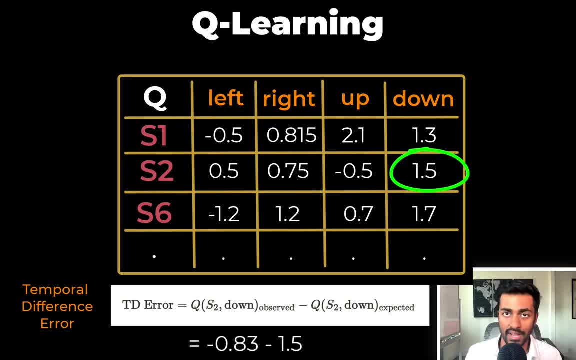 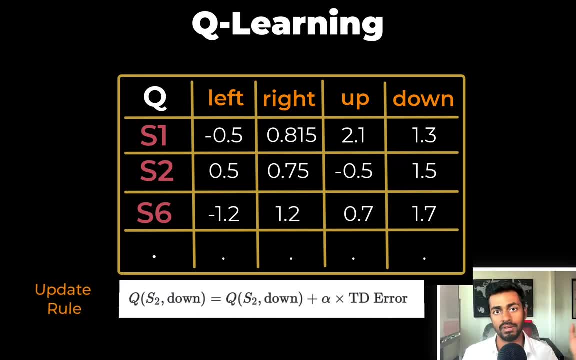 the observed minus the expected, negative 0.83 minus 1.5, and we'll get negative 2.33.. And now we're going to now plug this value into our update rule for the temporal difference error, And so this gives us a 1.5 for the current Q value expected plus 0.1 times the temporal. 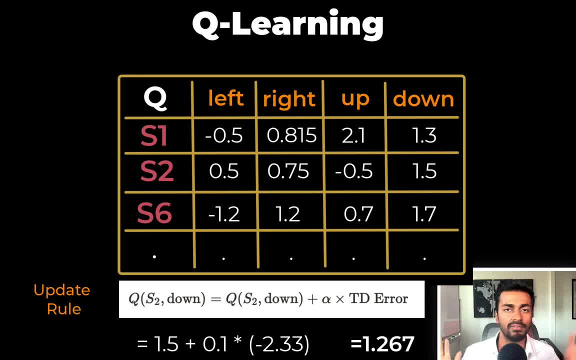 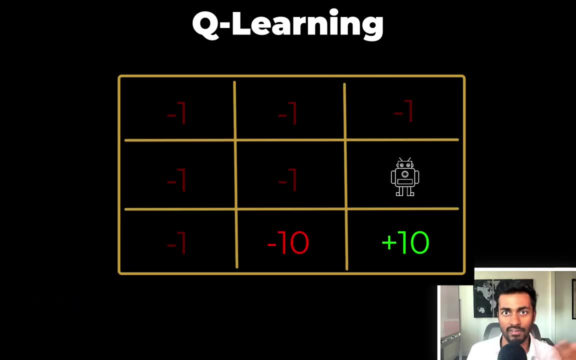 difference error of negative 2.33.. Doing the math, you get 1.267.. And so we update the single Q value in our table. And this is the end of our second time step. We repeat this until the sequence of steps is over, That is, until we get to the plus 10 spot. 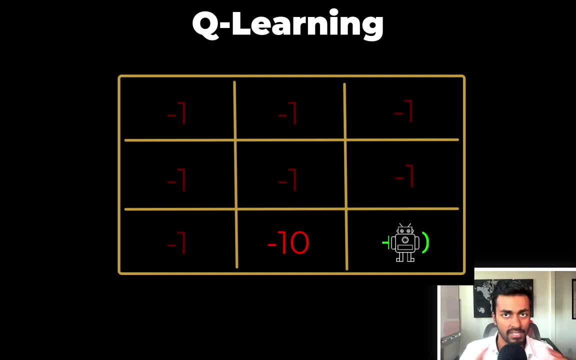 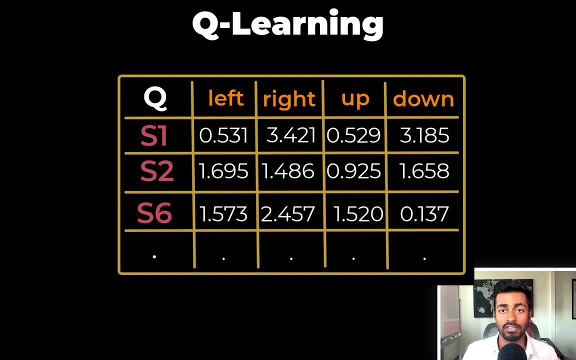 or the negative 10 spot, And this sequence of steps until now is known as one episode. We can then perform multiple episodes over and over again, choosing random actions and effectively just learning the values of the Q table until they become more stable And effectively these Q values are learned And once they are learned an agent can take an. 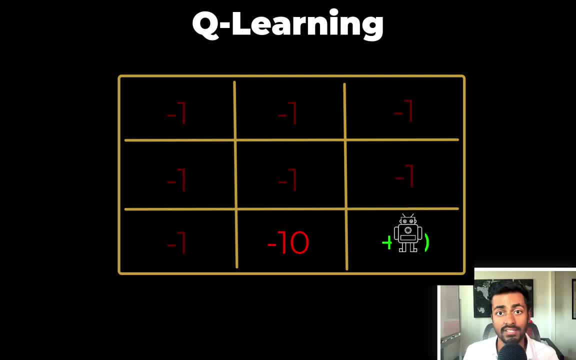 action based on which will give us the highest Q value results, And so the Q value will dictate the policy to get our reward. And this new policy, remember, was the target policy that we were trying to achieve, And note that this is different from the behavior policy that we use to explore.